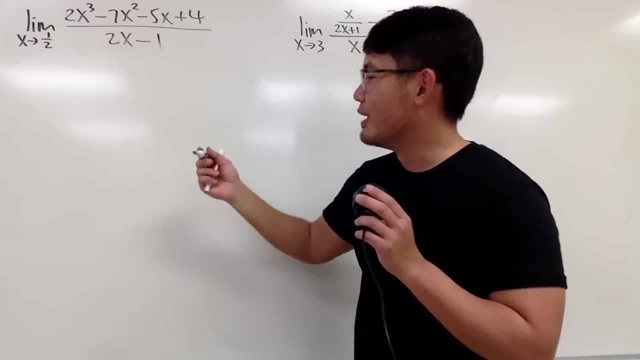 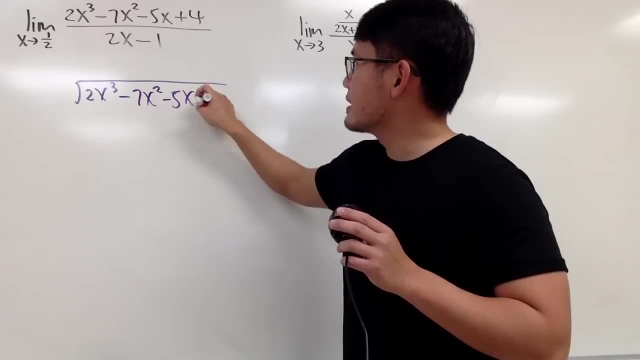 It's okay because we can just do polynomial divisions right here. So I'll do a long division right here which is 2x cubed minus 7x squared minus 5x plus 4.. And then on the other side I'll put down 2x minus 1.. 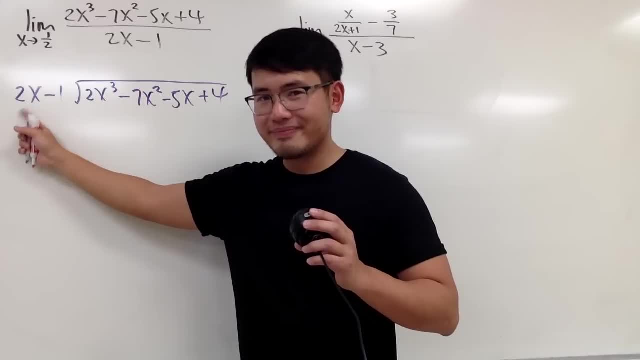 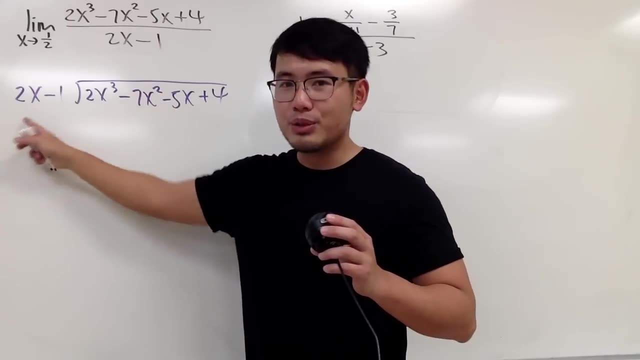 And here we go. So compare the first term with the first term. right here You have to ask yourself what times 2x will give us 2x to the third power. We know 1 times 2 is 2, and then we know x squared times x is going to give us x to the third power. 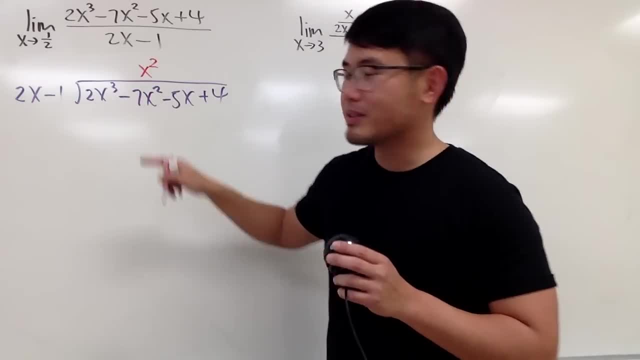 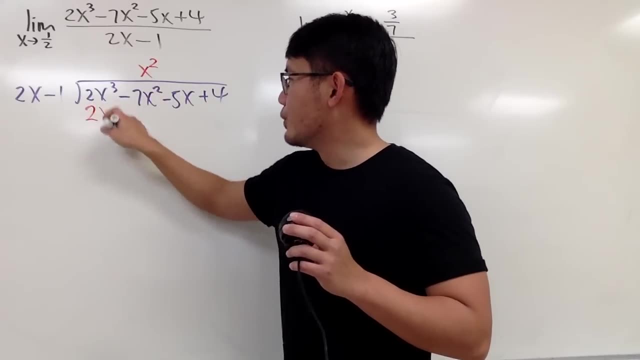 Therefore, I need x squared right. So you find out the x squared term right here. Now multiply x squared with 2x. We end up with 2x to the third power. And don't forget to do 2x times. 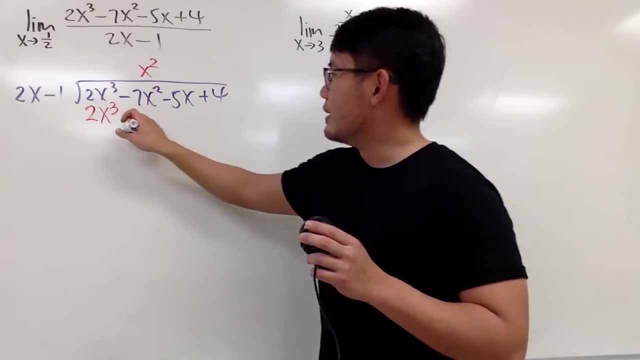 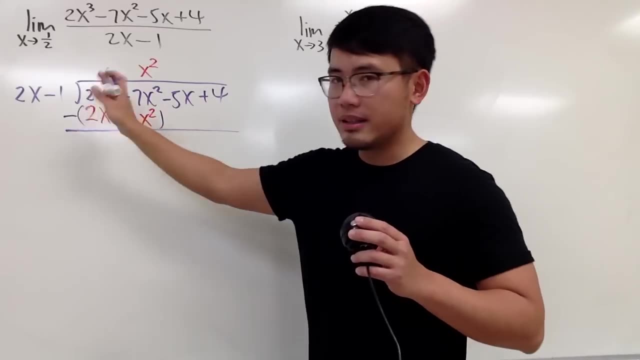 Don't forget to do x squared times minus 1, which is negative, x squared like this: And then for long division, of course, you subtract, and then be sure you put a minus in the parentheses, like this: Okay, this minus, that cancel. 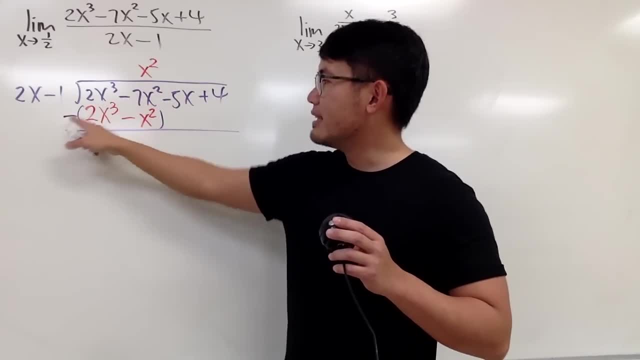 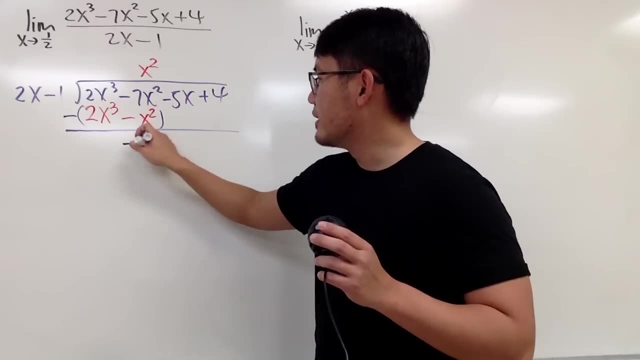 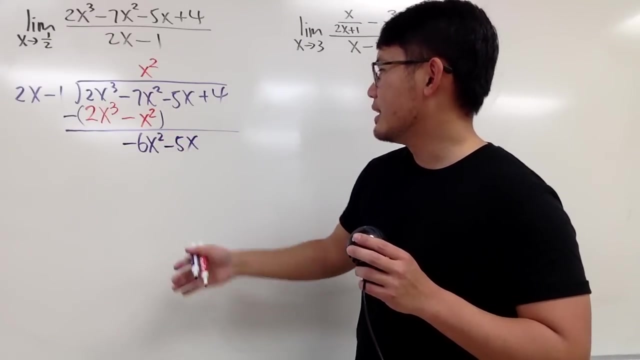 Next, negative 7x squared minus minus. in another word, Negative 7x squared plus x squared. give us negative 6x, squared right, And then we continue. This is minus 5x, and this time compare this and that. 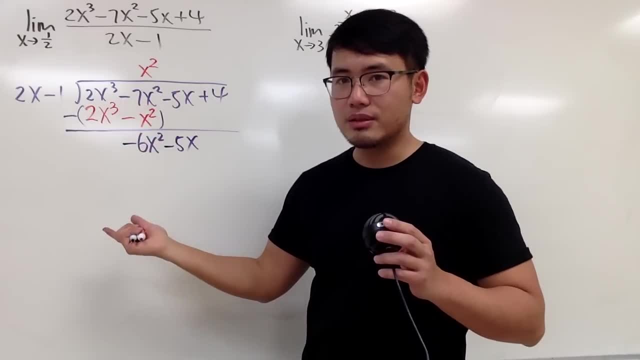 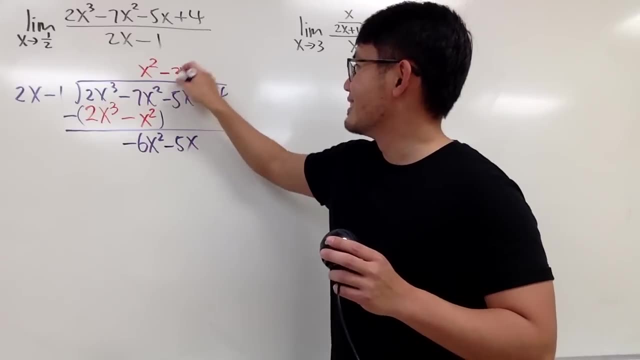 What do we need? What times 2 is negative? 6? That's negative 3,, right. And then what times x will give any x squared? I just need an x. So you take negative 3x times 2x. 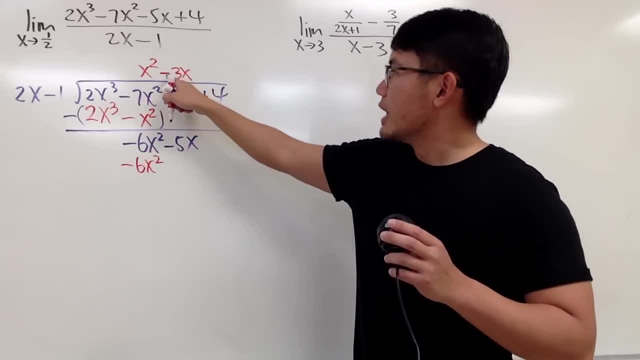 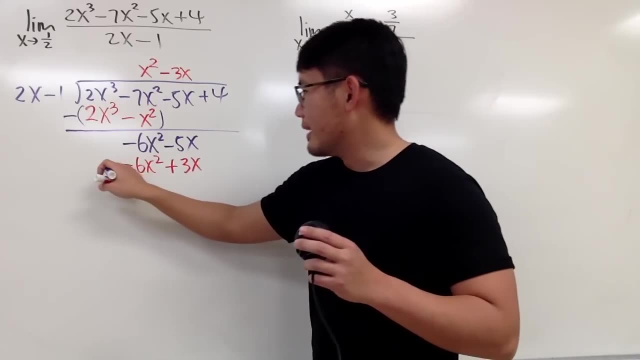 We end up negative 6x squared And then negative 3x times negative 1. give us positive 3x, like this, And then once again subtract. you put a parentheses like this: Now this minus that they're gone. 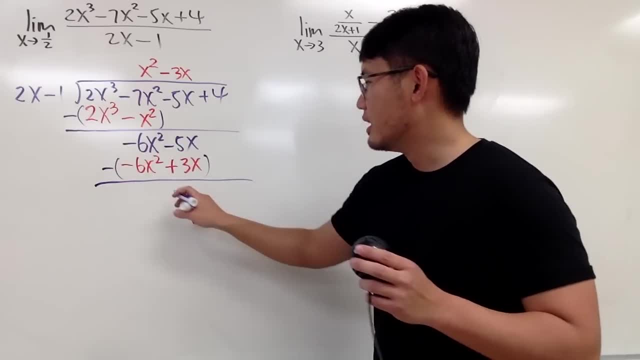 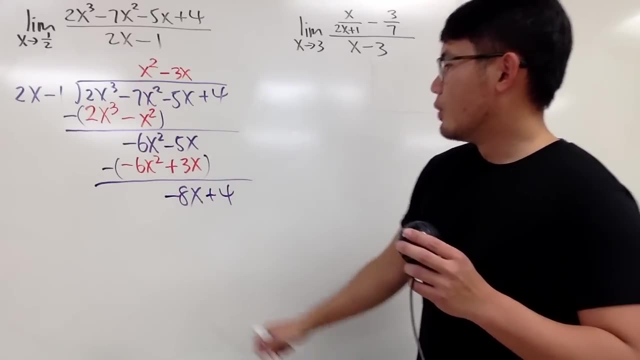 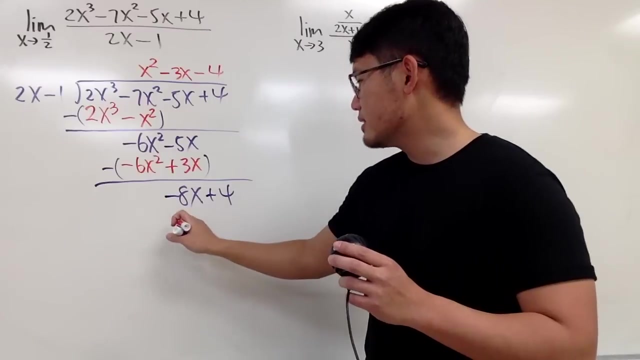 Negative 5x minus 3x give us negative 8x. And then you put this down, so you put down plus 4.. Well, what do I need next? Seems that I just need a negative 4, because negative 4 times 2x give us negative 8x. 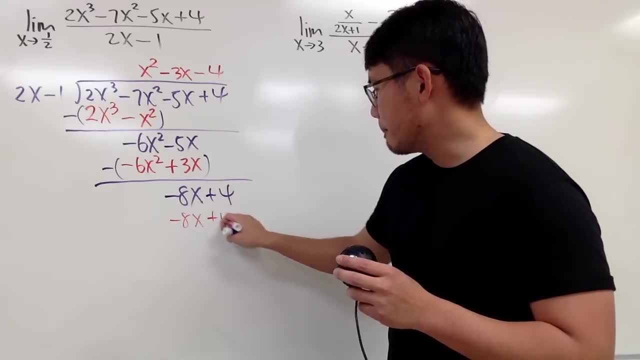 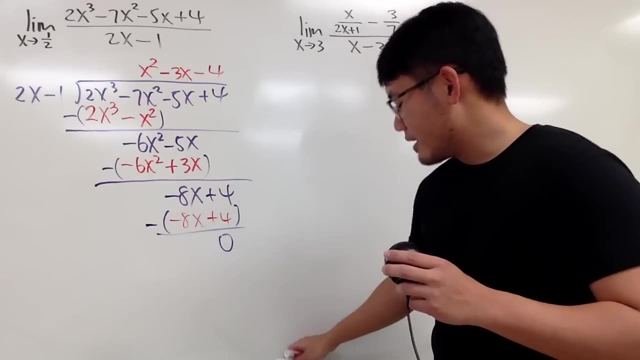 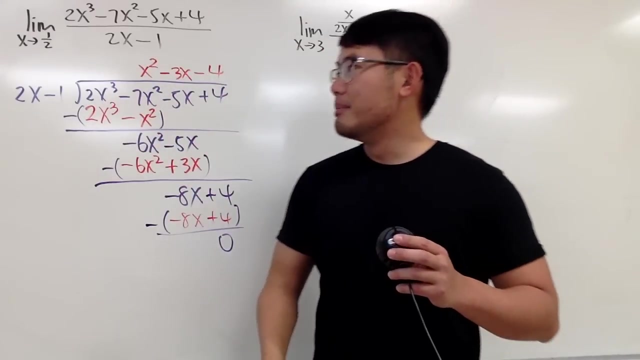 Negative 4 times negative, 1 gives us positive 4.. When you subtract this time it's 0.. So in another word, this right here all simplifies to this Namely x squared minus 3x minus 4.. 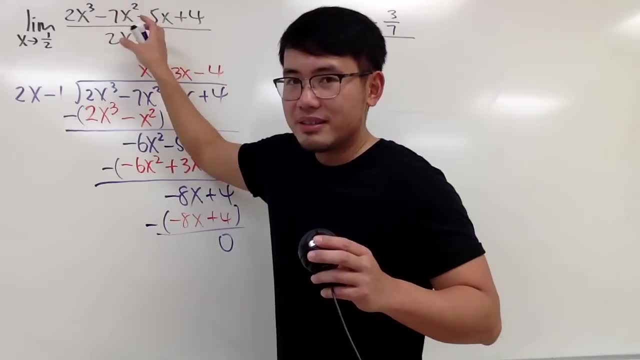 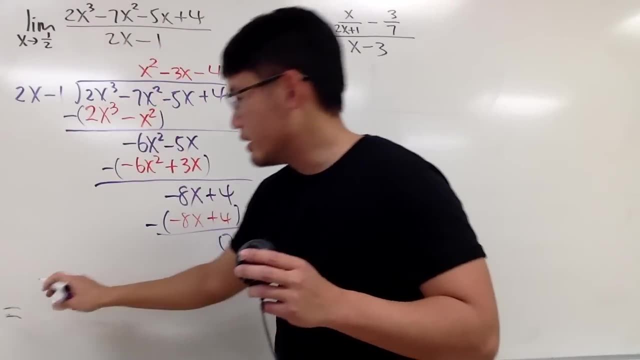 And you don't have to factor this anymore because, once again, when you divide this out, this right here is the result. So let me put this down. This original equation is equal to The limit as x, approaching 1 half of just this. 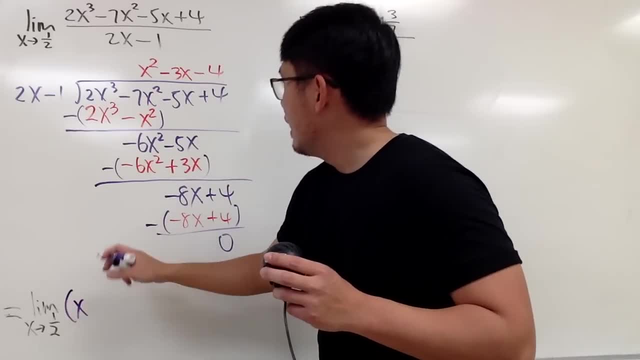 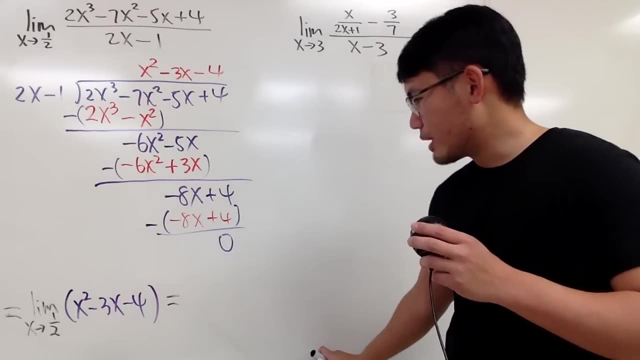 Namely. I'll just put this down in purple: x, squared minus 3x minus 4, right, Well, now you're going to put down 1 half into all the x. So let's see, We have 1 half and you square that. 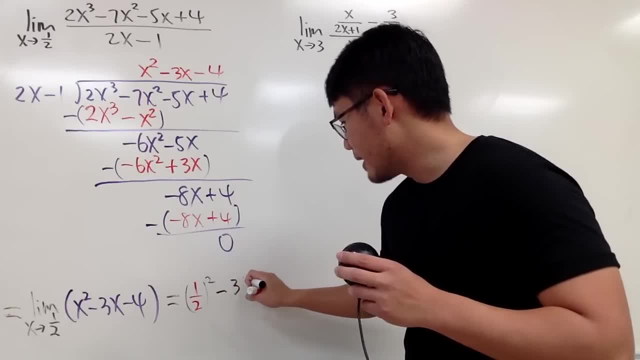 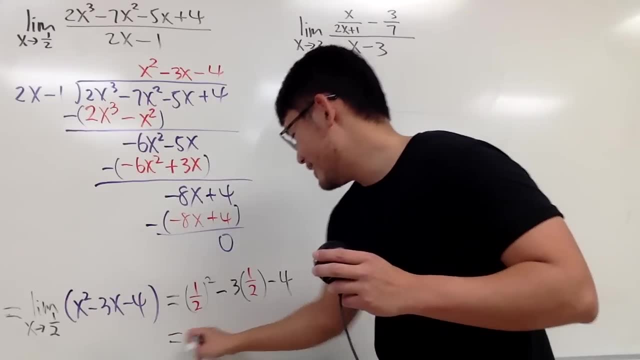 Minus 3 half. pretty much right. Minus 3 times 1 half And then minus 4, like that. Do this on your own Or do this in your head. let's see This is 1 over 4.. 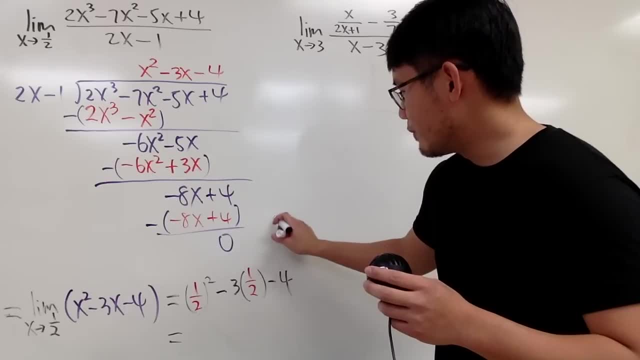 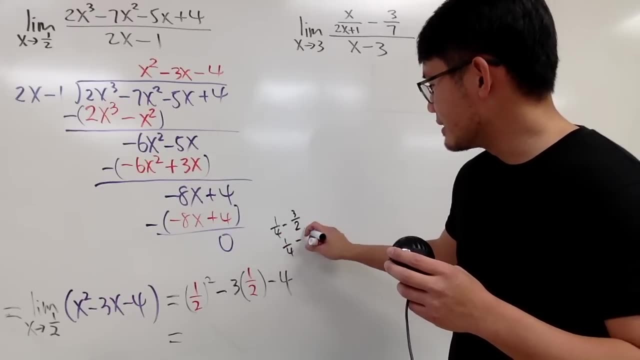 This is negative 3 over 2.. So if you have 1 over 4 minus 3 over 2, get the common denominator, So it's 1 over 4 minus 6 over 4.. So in another word, this is negative 5 over 4, together. 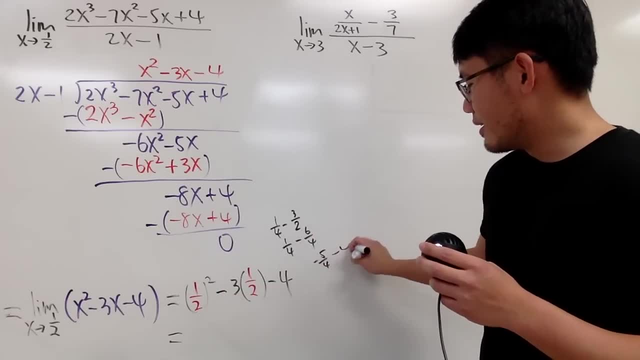 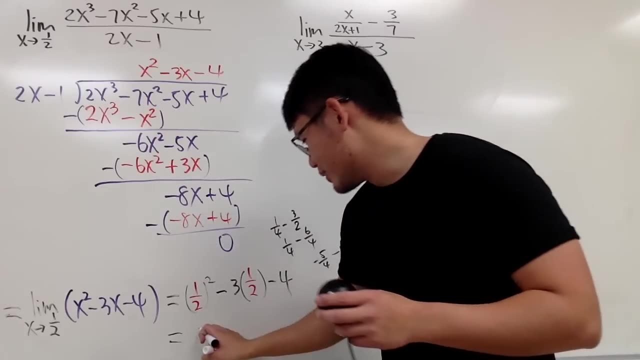 So negative, 5 over 4, right, And then minus 4. Which is the same thing as minus 16 over 4.. So this and that is minus 21 over 4.. So just do the fraction on your own. 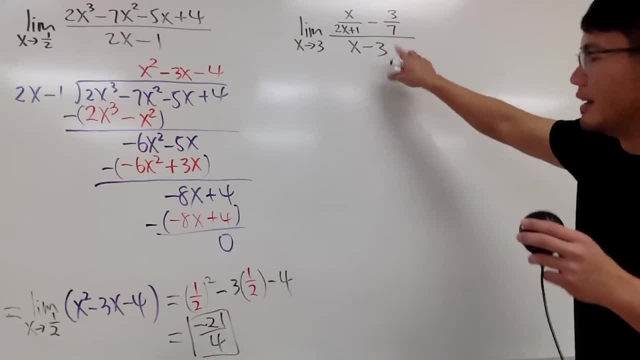 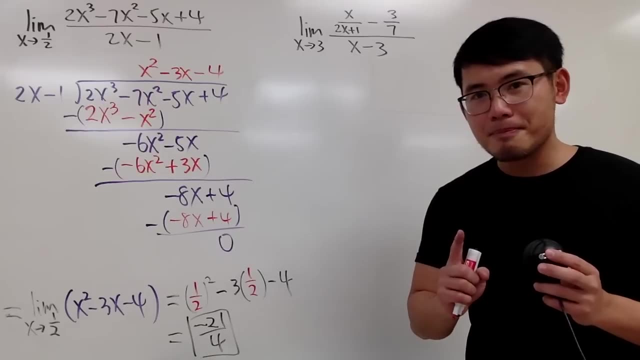 Right, Right Now. another one, right here. It's also: We need a lot of algebra for this. Yes, you end up with 0 over 0.. This time you have a complex fraction, So this is what you can do. 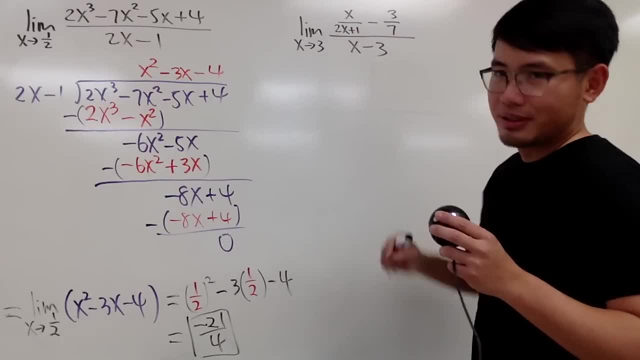 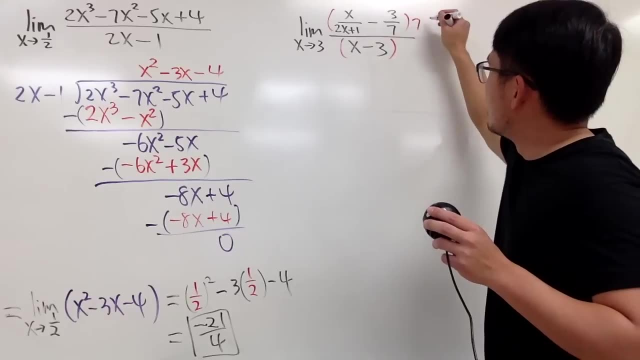 Denominator here. Denominator here: 2x plus 1, and then also 7.. There's no complex, There's no common factor. Go ahead, multiply the top and bottom by 7, and also the 2x plus 1.. 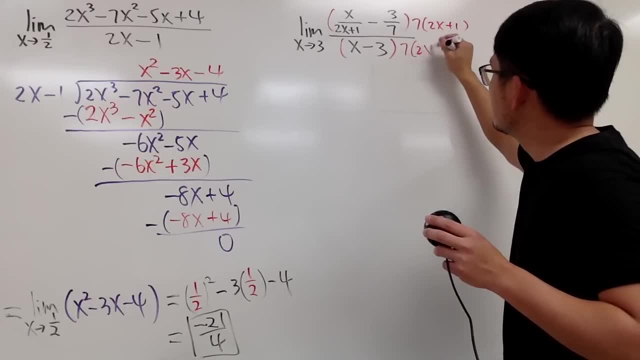 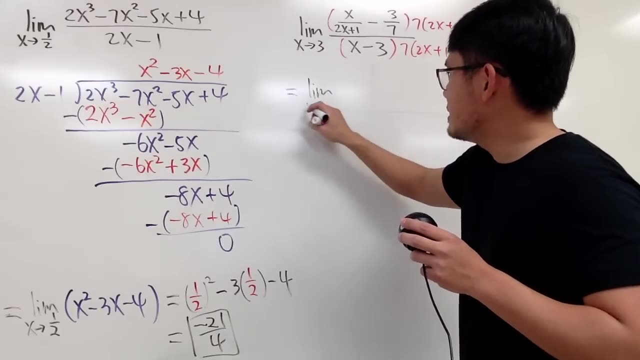 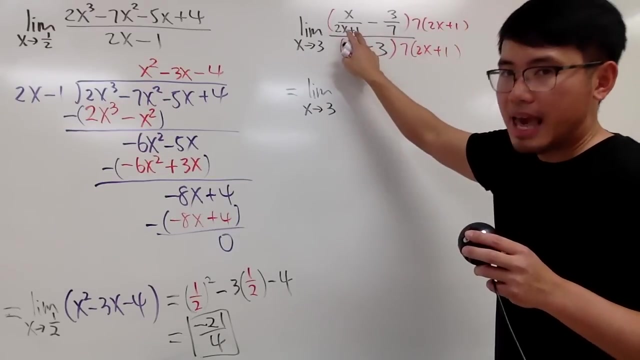 So multiply by the lowest common denominator of the small fractions And good things will happen. Just trust me. All right, Here we have the limit as x approaching 3.. When you take this, times that the 2x plus 1 cancel.